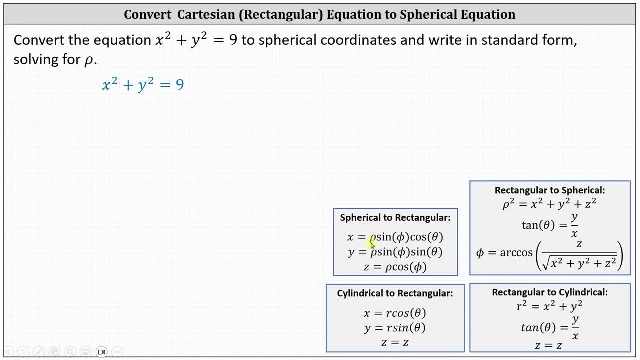 let's substitute rho sine phi cosine theta for x and rho sine phi sine theta for y. And now we'll go ahead and square. Now, comparing these two products on the left, the greatest common factor is rho squared sine squared phi. Let's go ahead and factor. 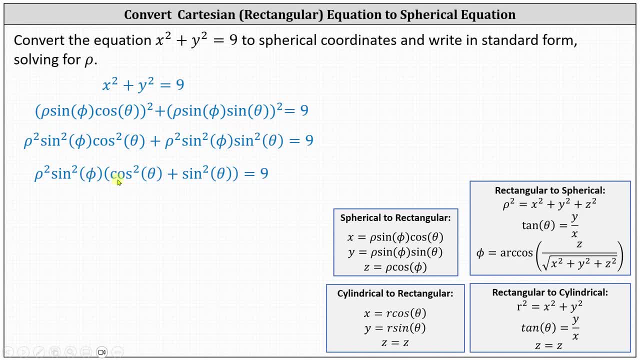 This gives us rho squared sine phi times the quantity cosine squared theta plus sine squared theta equals nine. And again using our trig identities, we know: cosine squared theta plus sine squared theta equals one. And now we'll divide both sides by sine squared phi. 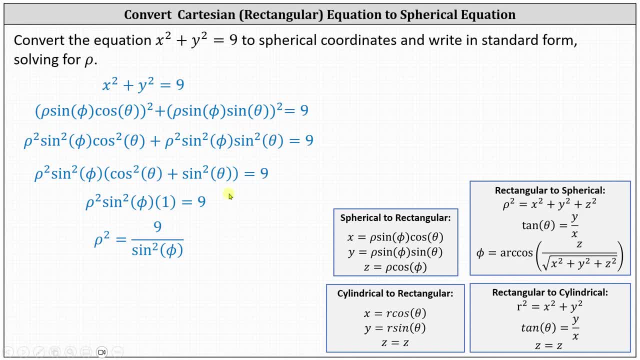 giving us rho squared equals nine divided by sine squared phi, phi. and once again we now take the square root of both sides of the equation, which gives us rho equals plus or minus 3 divided by sine phi. and again using the positive value, we have rho equals. 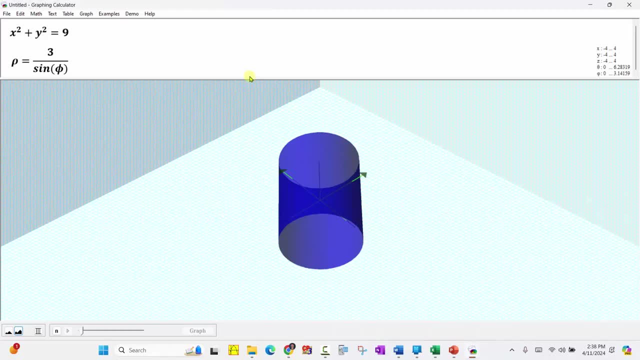 3 divided by sine phi. And now let's go ahead and check this graphically. In blue we have the graph of x squared plus y squared equals 9 in 3d, which gives us the cylinder. and now we'll graph: rho equals 3 divided by sine phi. Let's go ahead and graph that in red and the two cylinders should: 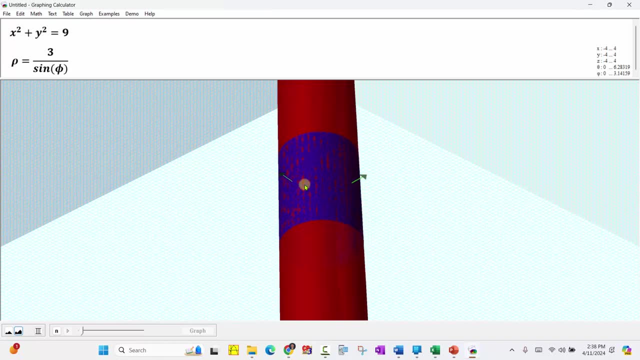 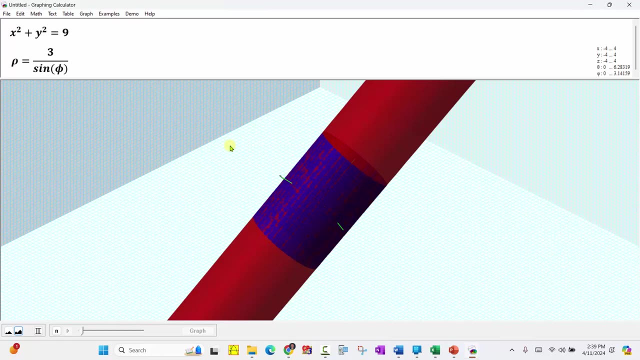 overlap and we can see they do. This verifies our work is correct. I hope you found this helpful. 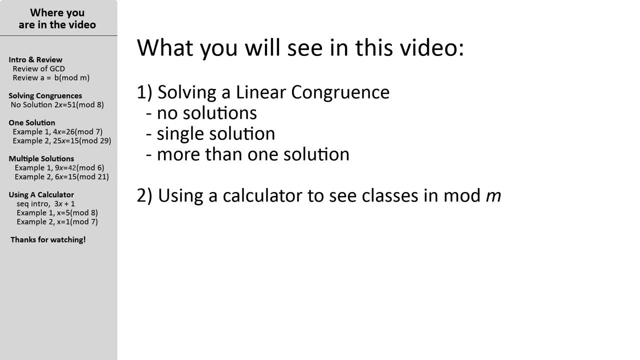 Hey there, YouTube viewer. This video will show you two things: The basic technique of solving linear congruences and how to use a Texas Instruments graphing calculator to help you generate congruence classes of modulo m. Before we dive into it, it's important. 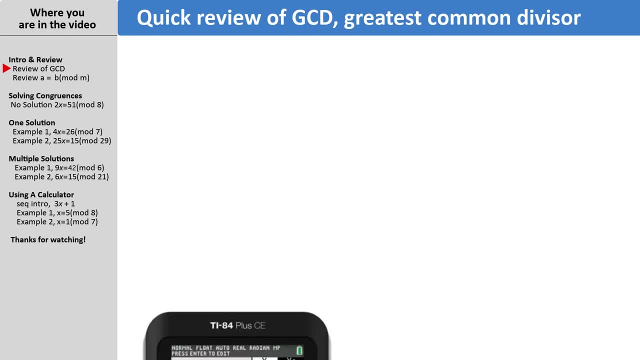 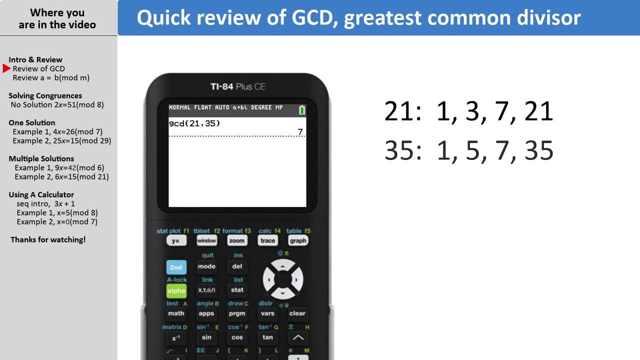 you have a solid understanding of greatest common divisor. Some calculators have built-in functionality for finding the GCD. If it's been a while since you've seen GCD, then simply find all the factors of both numbers, line them up side by side and identify the greatest.